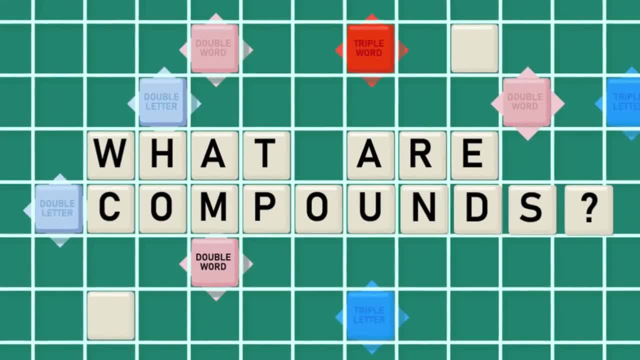 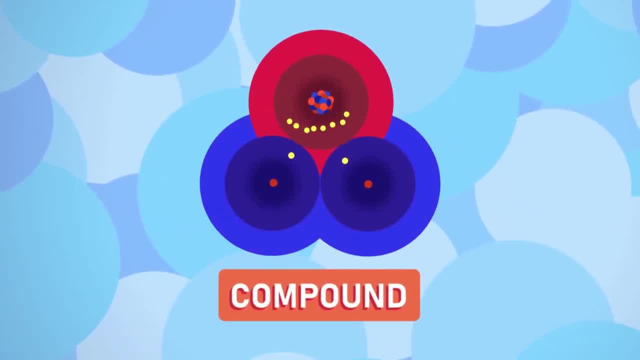 denoted as O3.. What are compounds? Remember how molecules are two or more atoms that combine together. Compounds are all atoms. What are compounds? Remember how molecules are two or more atoms. Remember how Cher trapene is also a molecule, but those elements must be different. 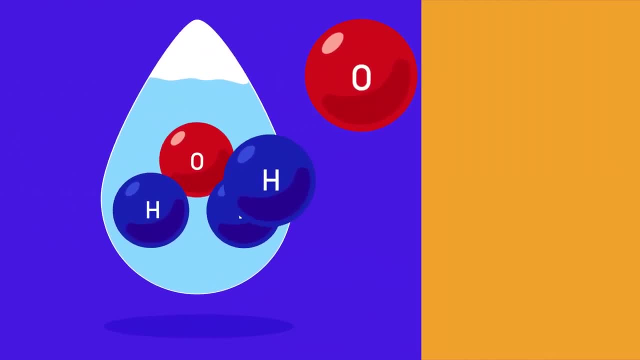 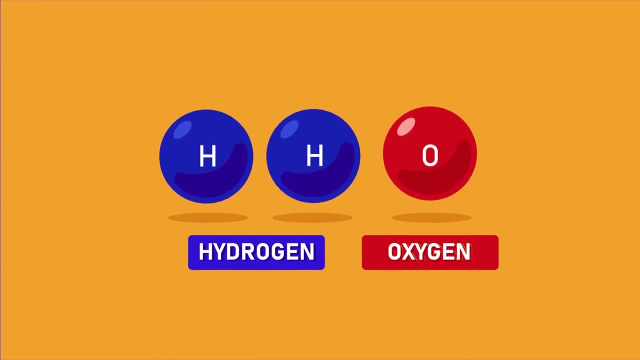 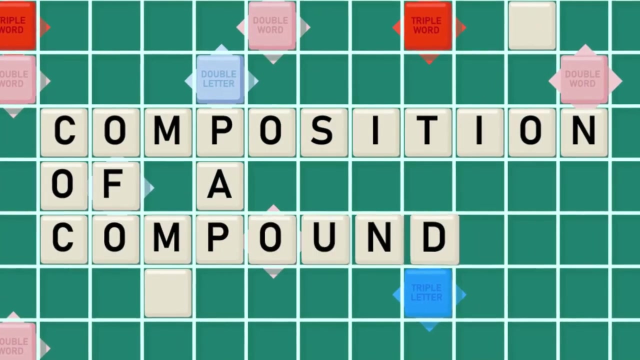 For example, water is a compound. It is made by chemically joining an oxygen atom with two hydrogen atoms. The ratio of hydrogen atoms to oxygen atoms in water is 2 to 1.. Changing this ratio will give us a different compound Composition of a compound. When we take a look at 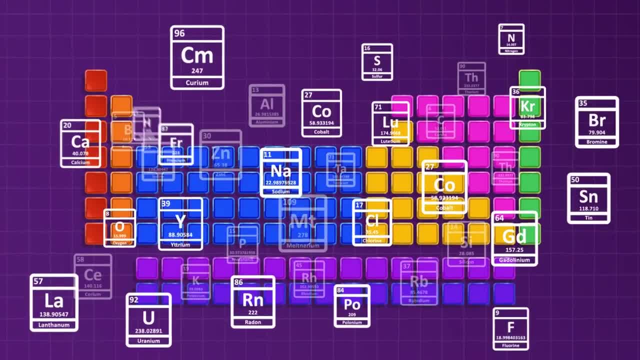 the periodic table, we find that all of the elements that make up the compound can be classified as metal and non-metal elements. This is what I call a component, because there are no choking elements in Business提icos. Then we will break it down to biorem and tear away its fairy-tolen gluten molecules. 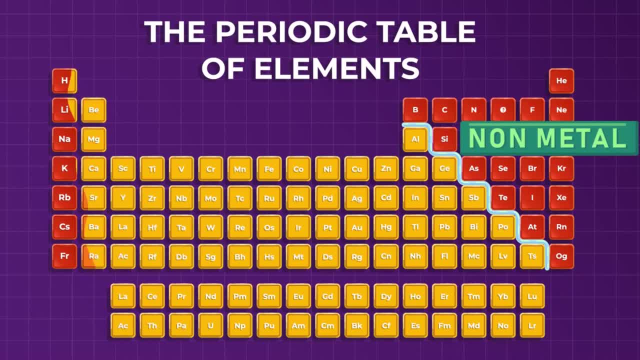 and immediately convert it to exist. If there are missed components in your new models, then we think that the compounds can be called H2O. When we convert the making, we will have trillion- standard. The right side of the line are nonmetals and the other side are metals except hydrogen. 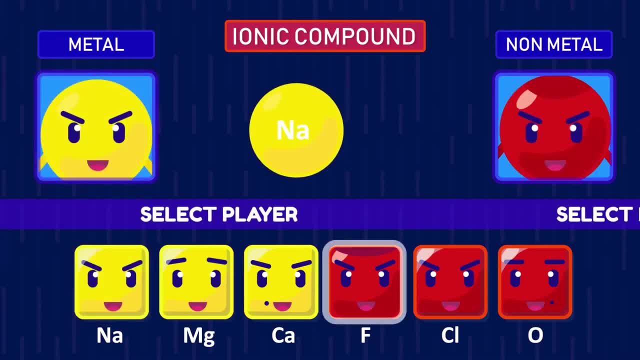 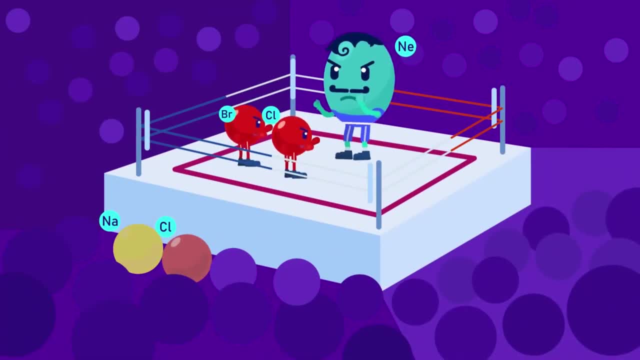 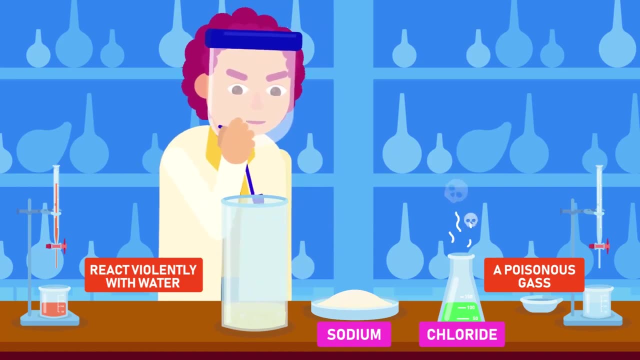 If metal elements are present to form a compound, it is called an ion compound. Meanwhile, if the compounds are only formed between nonmetallic elements, they are called molecular or covalent compounds. Properties of a compound. You may think that, since compounds are made, 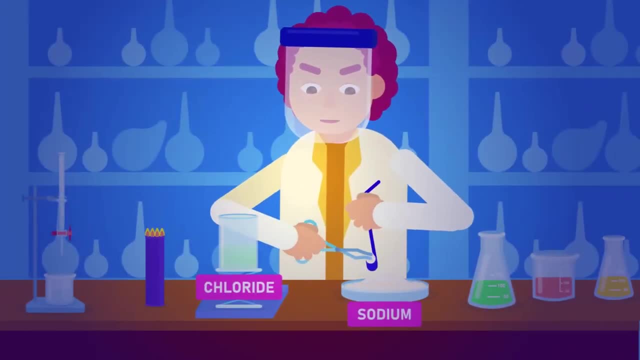 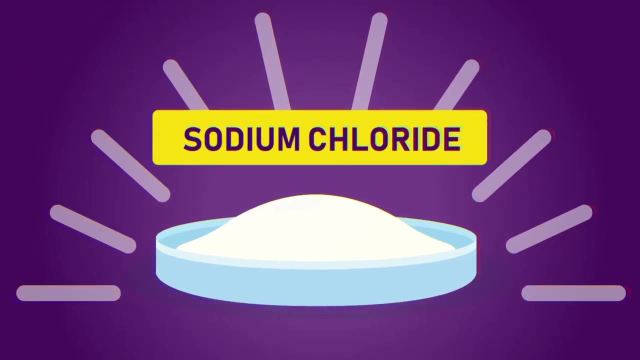 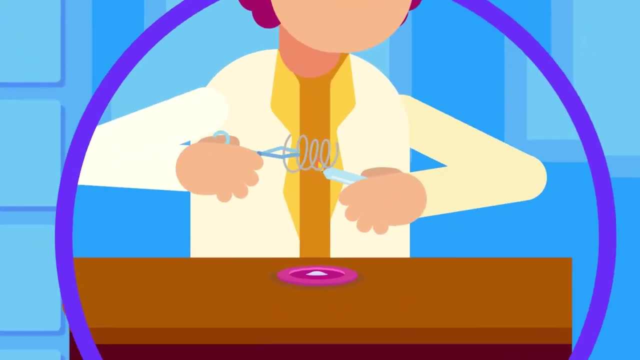 of elements combined together. therefore, compounds will have the same property as that of the elements that make it right. The fascinating thing is that this is not the case. A compound has different properties from the elements that form it. An example of this is that magnesium is a type of metal that burns in oxygen to form. 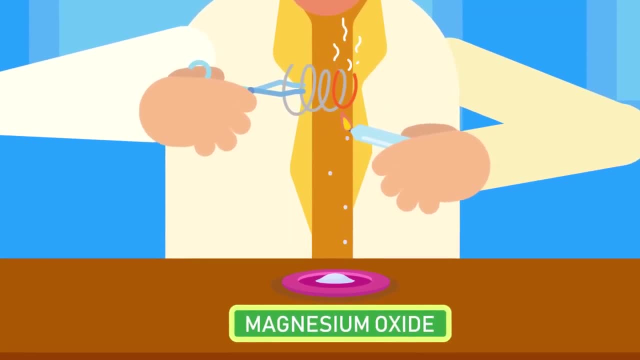 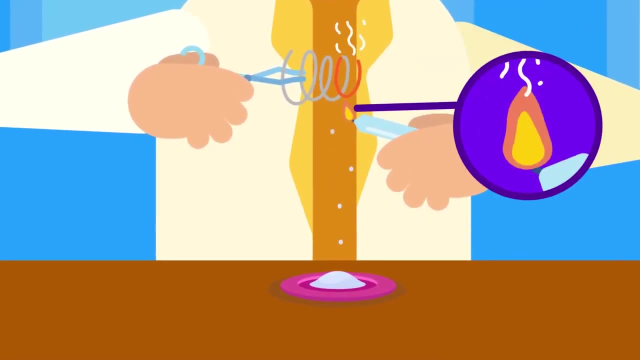 a compound called magnesium oxide. Magnesium oxide has different properties than both magnesium and oxygen. Magnesium is a solid with a silvery appearance. Oxygen, as we all know, is a colorless gas. However, magnesium oxide is a white gas. 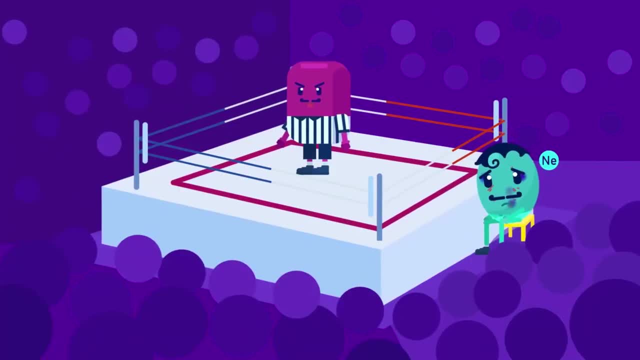 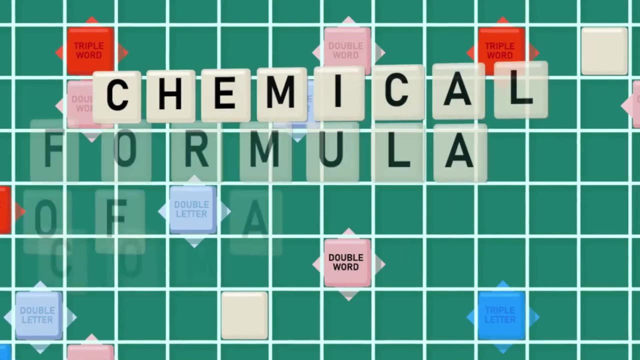 It is solid Naming compound. Naming compounds are relatively straightforward. For example, carbon and oxygen combine to form carbon dioxide. Sodium and chlorine chemically combine to make sodium, chloride And zinc, and oxygen form zinc oxide. Chemical formula of a compound. A chemical formula tells us the types of elements. 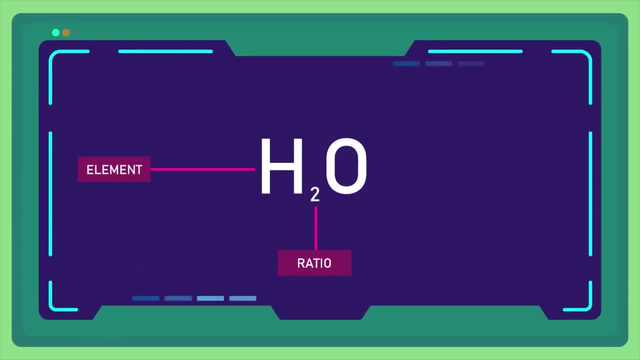 present in a compound and the ratio of different atoms present in a compound, For example H2O. The H and O tell us the ratio of H2O to H2O. The H and O tell us the ratio of H2O to H2O.